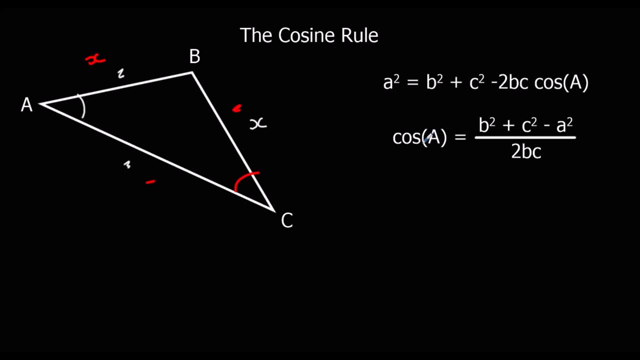 the angle in between them, Or I could find a missing angle when I know all three sides. Okay, this length. Let's look at an example Here. I've got find the length of AC, So this is X And. 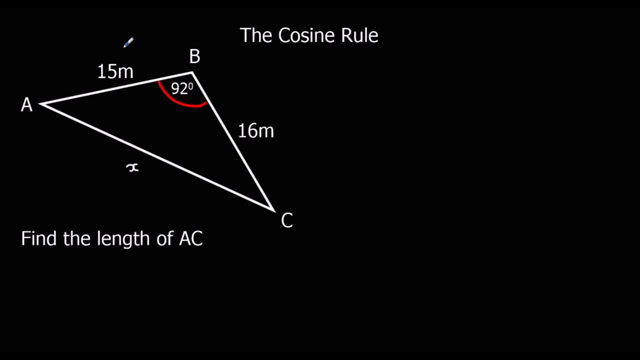 we can see. I've got an angle and the two sides next to it. That means it's a cosine rule question. The cosine rule to find the length is this: here A squared equals B squared plus C. squared minus 2BC cos A. So that's the length. 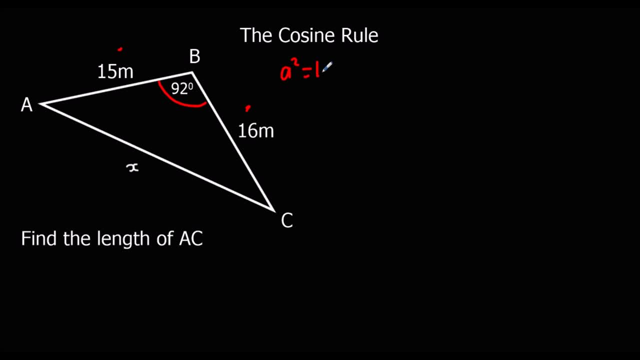 That's the formula I'm going to use. I'm going to use: A squared equals B squared plus C squared minus 2BC cos A. Now I want my A squared this, A here and this. well, I need this big. 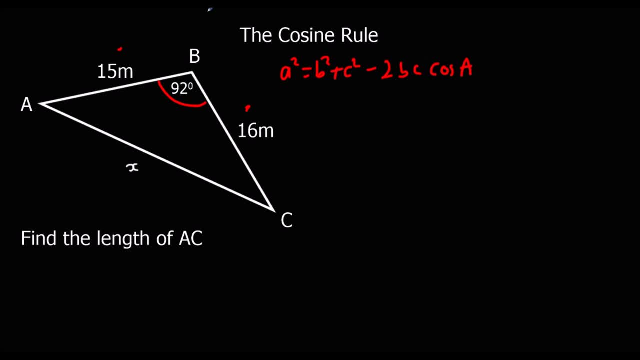 A to be the angle I know. So this big A is going to be here. 92 is going to be the big A. Little a is going to be opposite. So that's going to be little a, that's going to be big. 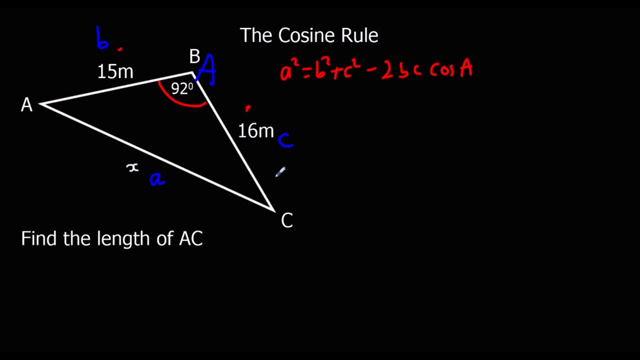 A And these two are going to be B and C. It doesn't matter which way around B and C you go, as long as they're the other two lengths. So now I can substitute my numbers in. So I've got X squared equals 15 squared. 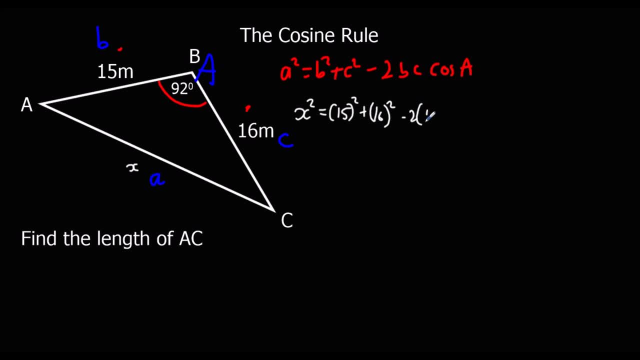 plus 16, squared minus 2 times 15 times 16, cos 92. Then I can type all of this in the calculator. So I can type: 15 squared plus 16, squared minus 2 times 15 times 16, cos 92. That can. 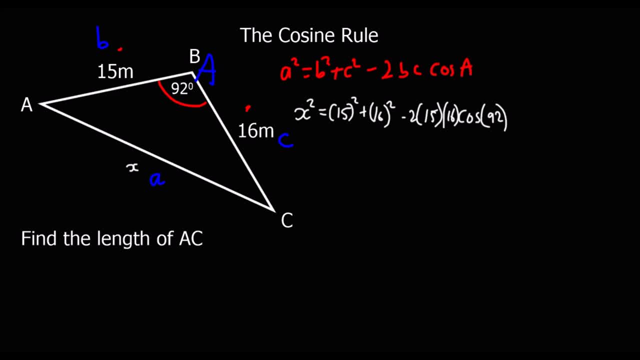 go in the calculator in one go. So I type that in the calculator and I'll get an answer out. The answer I get out will be quite a big number because it's X squared. So I get the answer out for X squared And then to get X from X squared I have to square root. 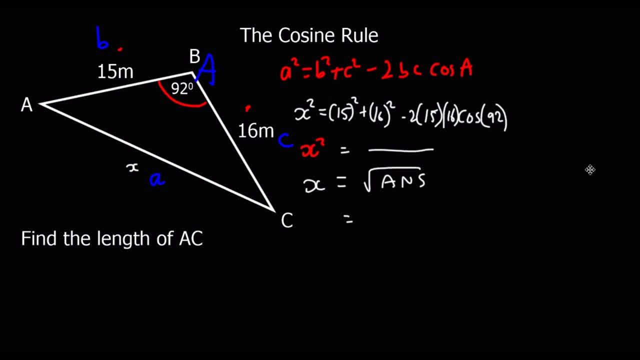 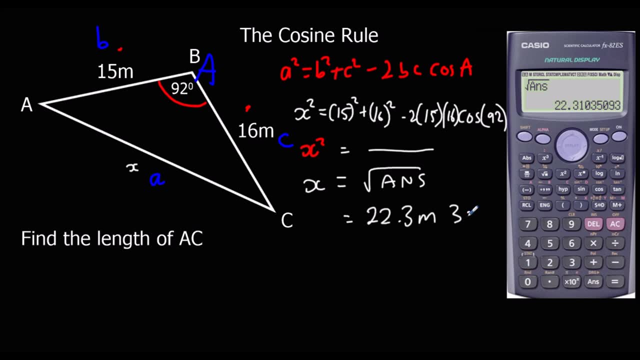 the answer. So in this example, square root the answer and I get 22.3 meters to three significant figures. So you type all of this in the calculator, get your answer and square root it And that gives you A. 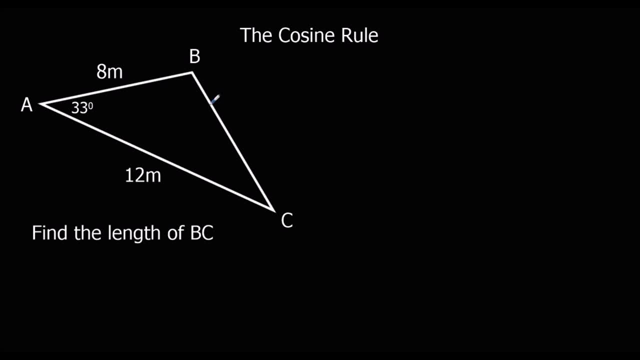 That's our missing length. So we do another example of that. So the length of B, C. So that's what we want to work out. We can see we've got two lengths and the angle in between them. it's a cosine rule question. So we write down the cosine rule to find the length. 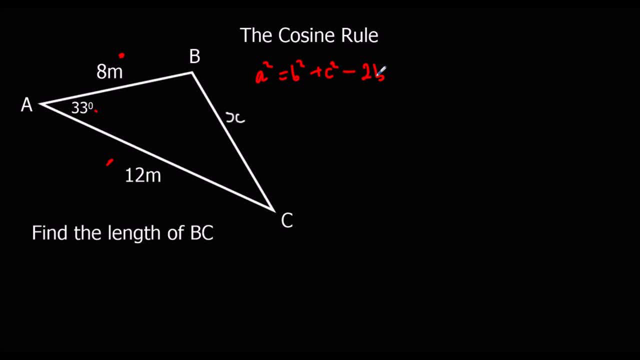 A squared equals B squared plus C squared minus 2BC cos A. We want big A to be the angle we know. So this is big A. opposite, it is little a and the other two are B and C. Then we can substitute the numbers in: So A squared is X squared equals posture. Then we can. 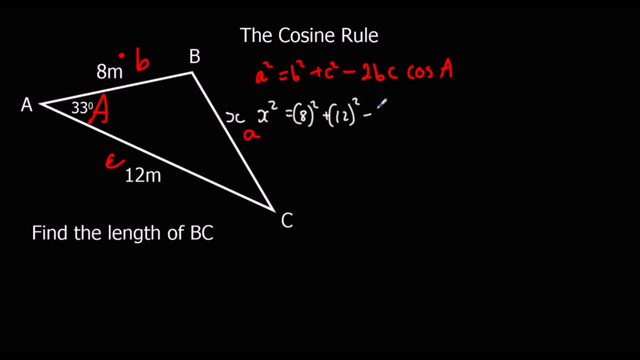 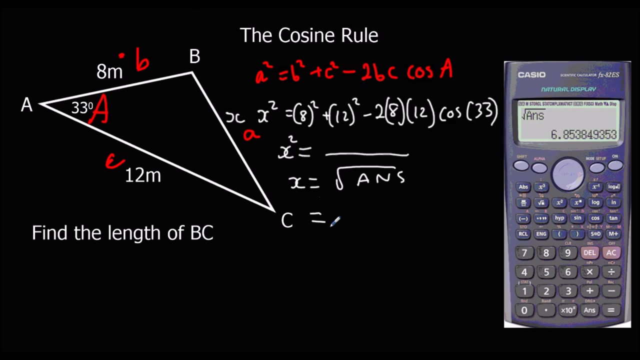 eight squared plus twelve squared minus two times eight times twelve, cos 33, then you type that in the calculator, you get your answer out for x squared and then you square root your answer and if we square root that answer we get 6.85. so 6.85 meters to three significant figures. 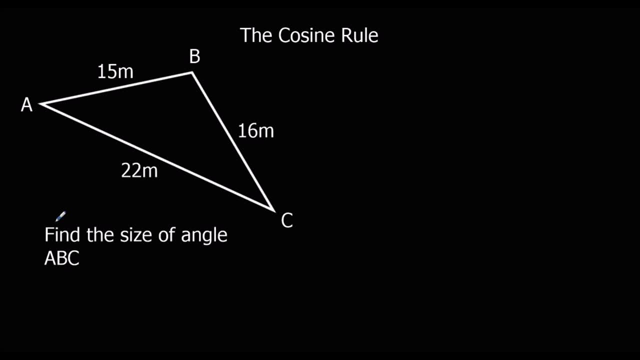 okay, now we're looking at an angle question, so find the size of angle a, b, c, a b c. that's here we know all three lengths. so it's a cosine rule question to find the length. so we have to write down the rule first. so cos a. 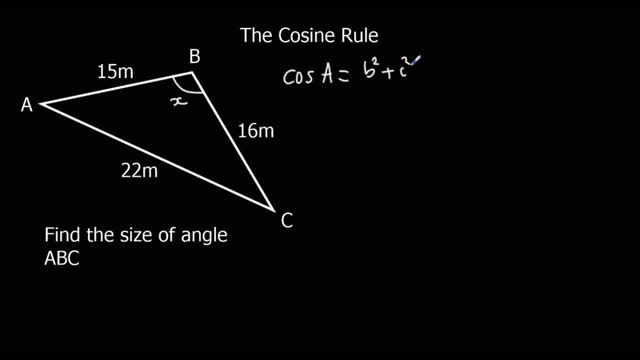 equals b squared plus c squared minus a squared over 2 b, c. now let's decide what a squared what a, b and c are. so the angle is going to be big a, so that's big a. opposite, it is little a and the other two are b and c. 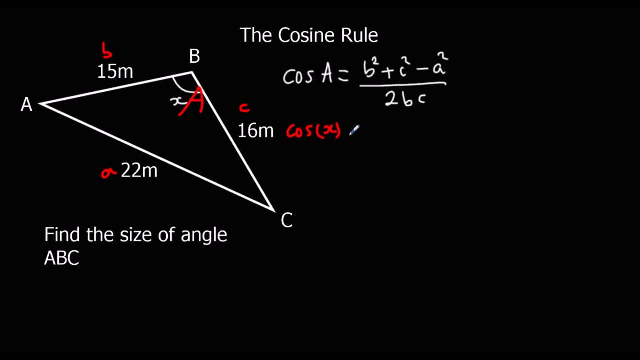 so now we've got cos x equals 15 squared plus 16 squared, minus 22 squared over 2, b, c, so 2 15, 16.. so now we type all of this side into the calculator, all of that goes into the calculator and we get an answer for cos x. 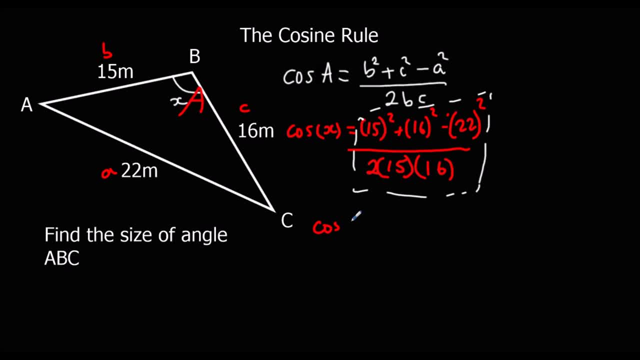 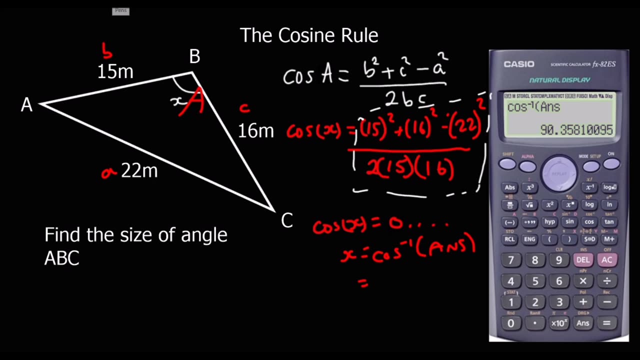 it'll be a decimal answer, so that'd be: cos x equals zero, point something. and then to get x by itself, we shift, cos, so shift cos the answer, and then we get our answer out, which is 90.4, 90.4 degrees to three significant figures. 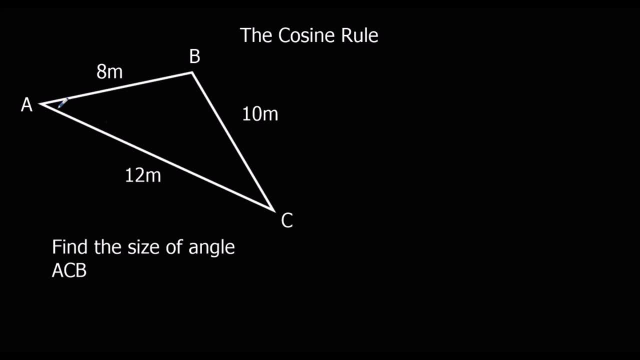 okay, another example of this. so acb, this time a, cb. that's over here and We'll write down the rule. So cos a equals b squared plus c squared minus a squared over 2bc, We need the angle x to be big A, So that's big A. Opposite, it is little a and the other two are b and c. 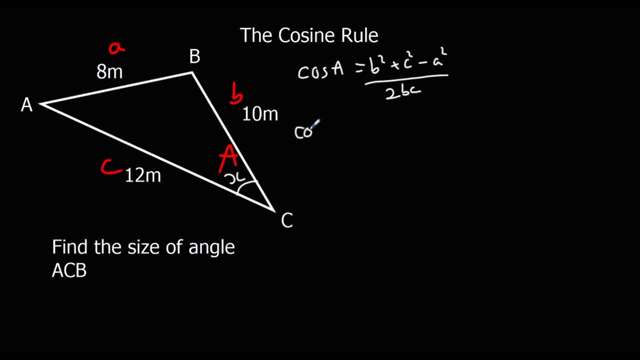 Now we substitute in. So we've got cos x equals 10 squared plus 12 squared minus 8 squared over 2 times 10 times 12.. Type that into the calculator and that gives you your answer for cos x. So again it'd be a decimal answer. And then we shift cos. 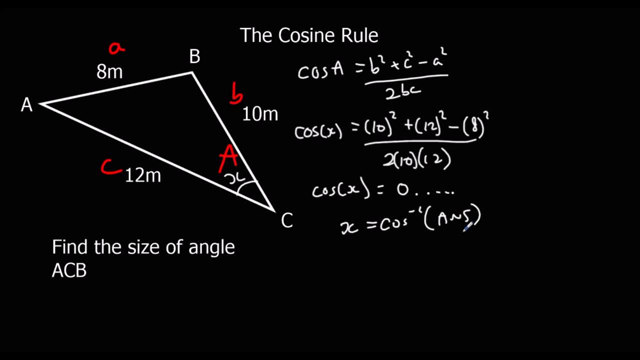 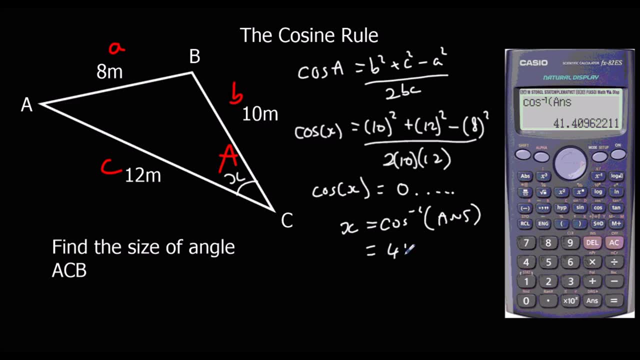 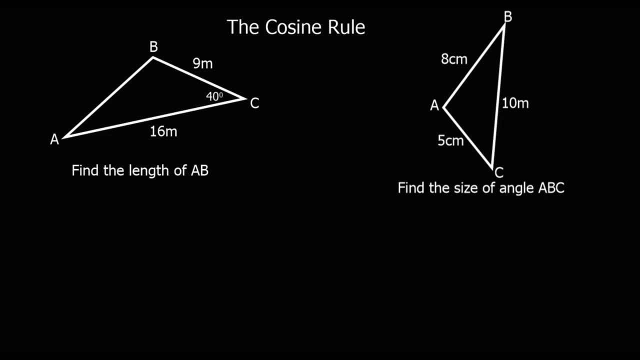 So shift cos that answer And we get out 41.4.. 41.4 degrees to three significant figures. OK, here's two for you to try. So pause the video and give them a go. OK, so the first one here is final length AB. That's here. 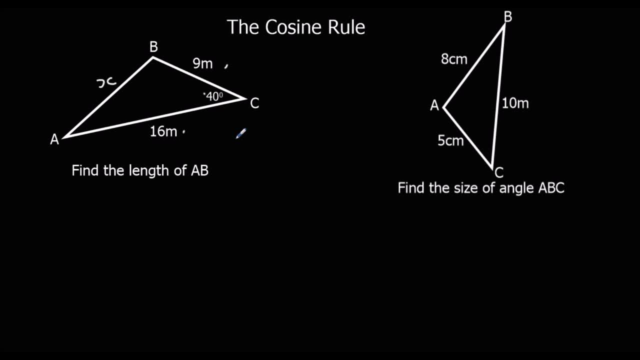 We've got The two lengths for an angle in between them. It's a cosine rule to find the length, So a squared equals b squared plus c squared minus 2bc cos a. We need Big A to be the angle, So this is big A. 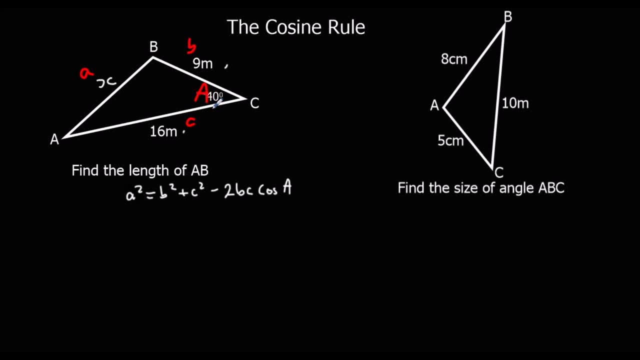 That's little a, and the other two are b and c. Now we substitute in, So we've got x squared equals nine squared Plus 16 squared, minus two times nine times 16, cos 40. We type all of this side into the calculator and we get our answer for x squared.